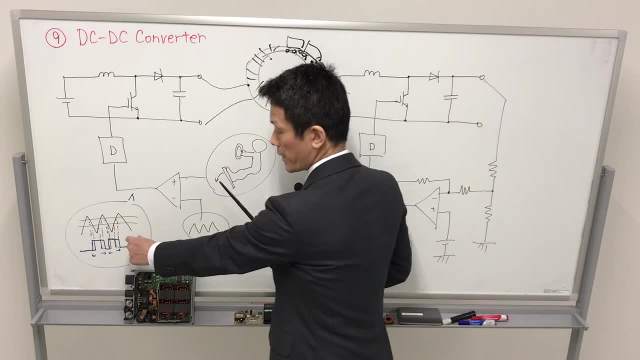 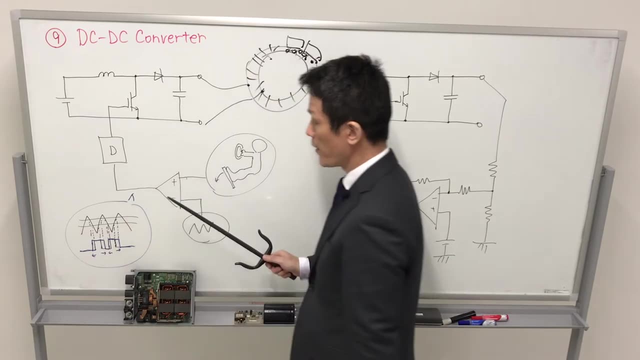 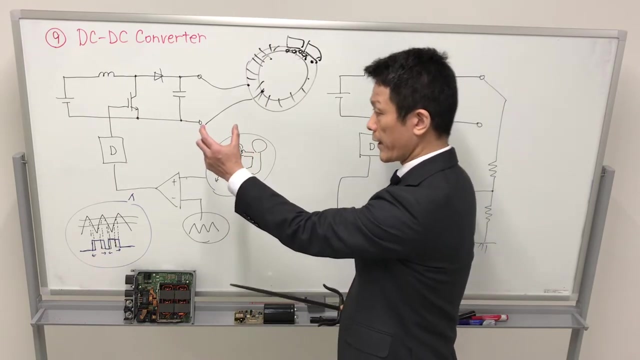 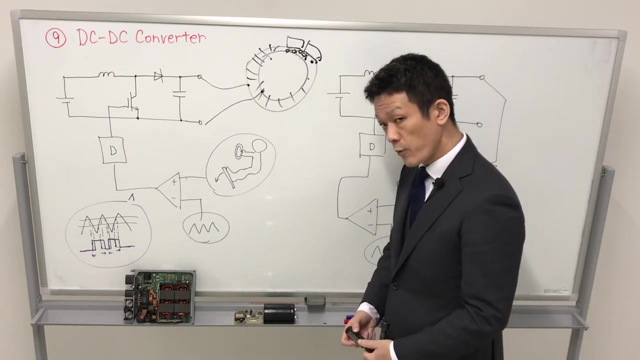 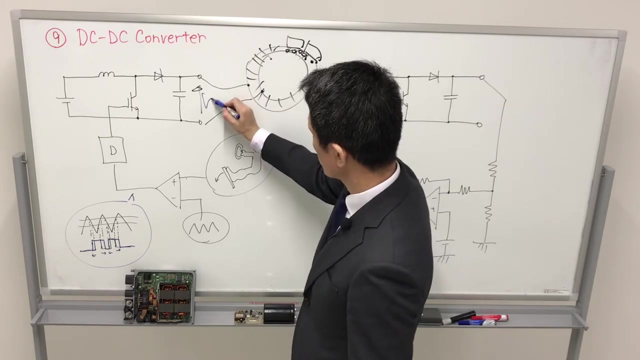 And we obtained the pulse width, increasing pulse width performance. And through the drive circuit we can obtain the wide width Pulse for the boost chopper. In case of the wide width boost chopper, output voltage, Output voltage, Vout and Vin. 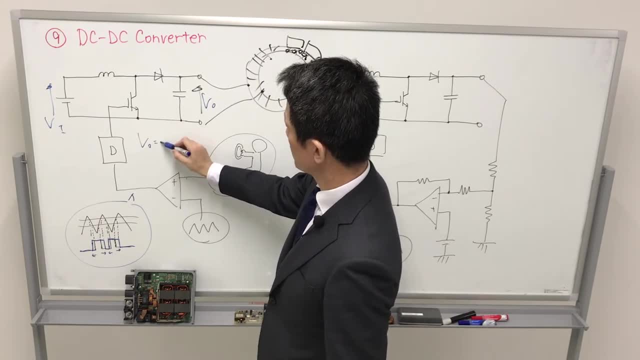 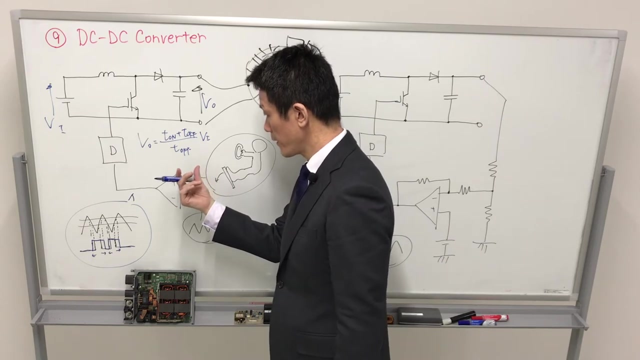 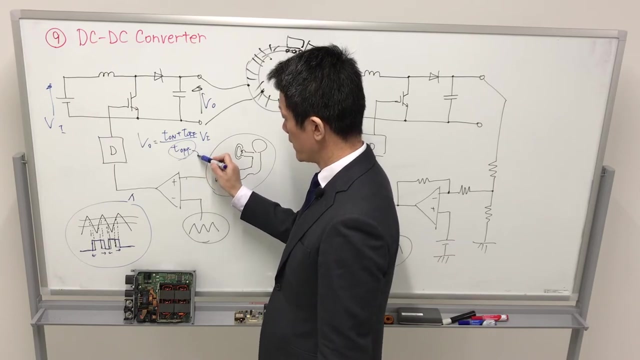 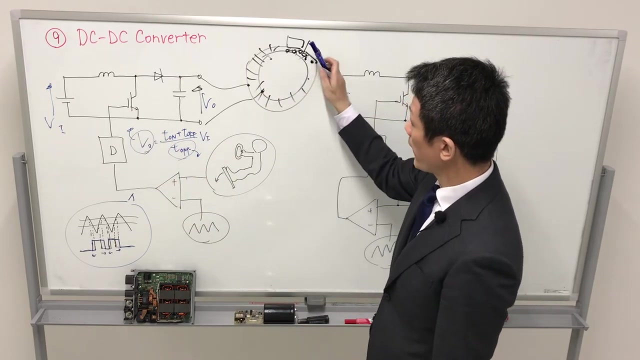 Vout equal to the T of term and Ton plus T of Vin, We can obtain this term. So in case of the term turn on term is increased, This T of term is decreased, So we can obtain the higher voltage. In case of the output voltage higher, the train speed is higher. 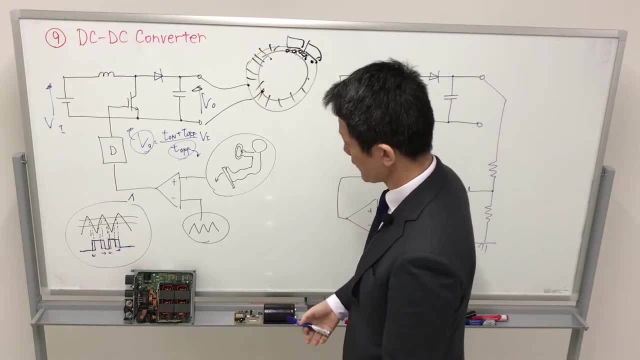 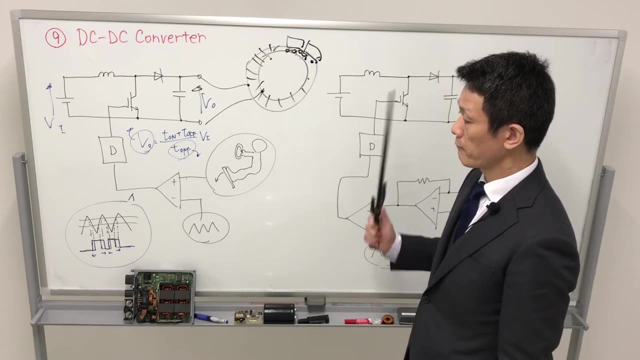 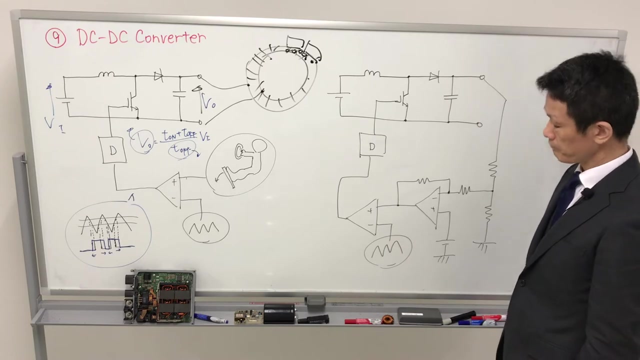 This is a very simple automotive applications For the Power Electronics, Accel Control Prism, only the prism. However, in the rear rear automotive application we have obtained, for example, this Ablis DTDC converter- We can control the motor drive. 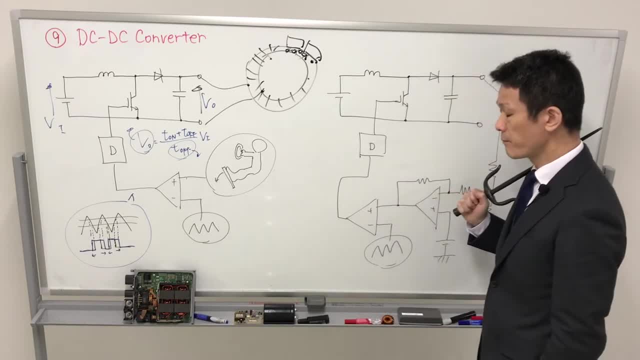 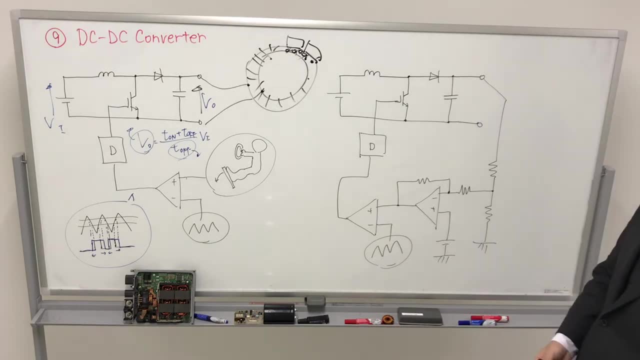 Motor drive is only applied for the AC drive, AC motors, So AC motors for the Japanese hybrid system is battery system, main battery system, DC-DC converter And obtain the higher voltage And through the inverter Inverter We can obtain the AC alternating current. 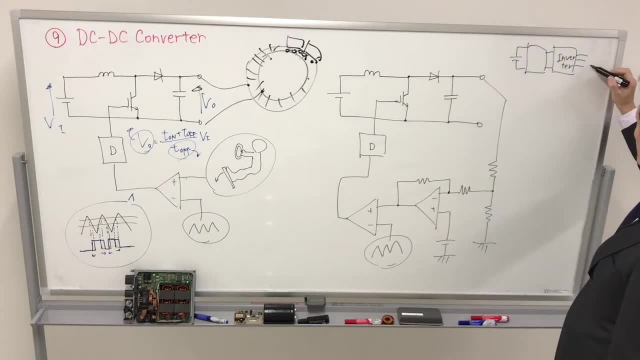 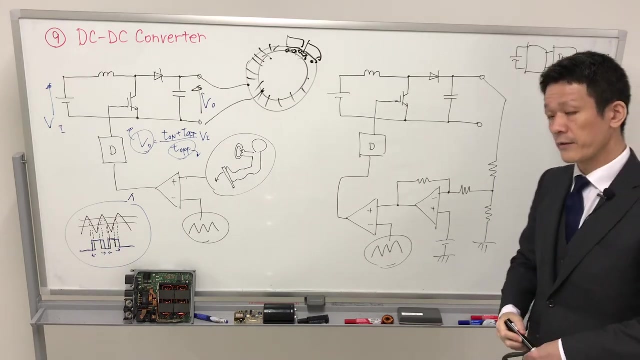 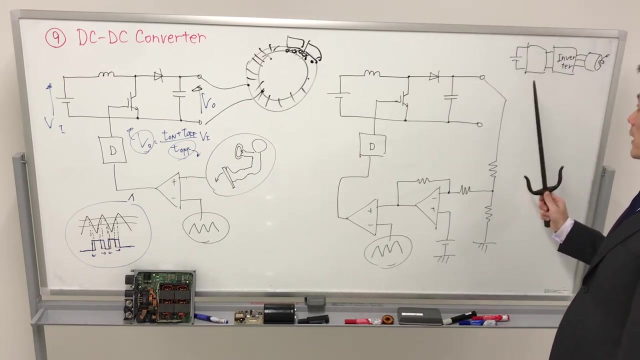 Output voltage current And we can drive the AC motor Because the output is 3-phase AC motor. So we can obtain the power Output power for driving by electric power, Boost chopper And inverter. This is the Prius and Yaris and some Toyota's famous. 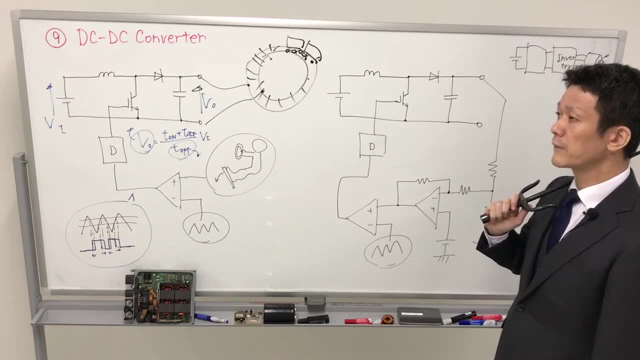 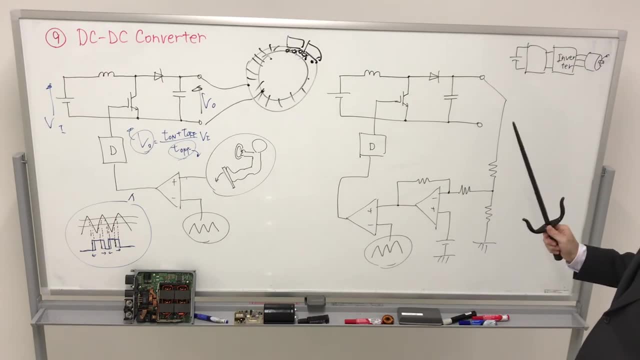 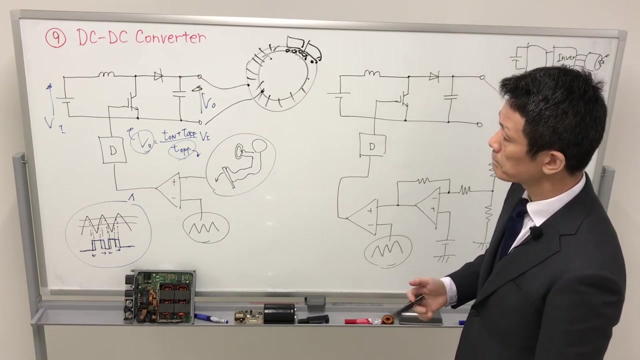 In case of the Honda is the Accord and fuel cell type quality. They have included the boost chopper and inverter. I mean this boost chopper Or, in case of the 48V, Mercedes S class And C class, Audi's SQ7.. 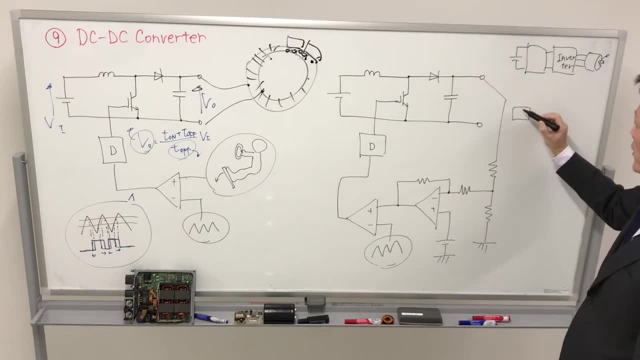 Some system have that Redux And DC-DC converter And 12V- 48V Ritual battery And using this inverter, Inverter And drive, We can obtain the electric power For driving Torque assist drive. 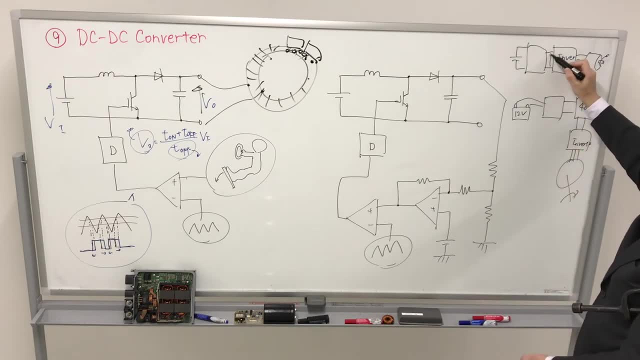 But, however, the In case of the Prius, The voltage is 600V. However, the, In case of the Europeans, Mild hybrid Electric system Is only driving for the Main, driving in the engine, Using the engine. So 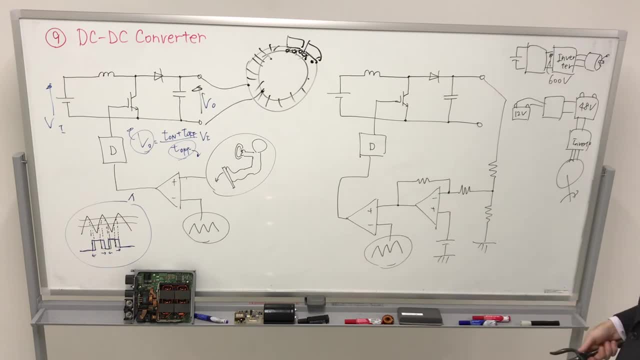 48V is torque assist, So The Around, the 10. To 12. Audi's one is 22.. Max power is 22kW. Motor driving. However, this, This type is Obtained higher voltage. 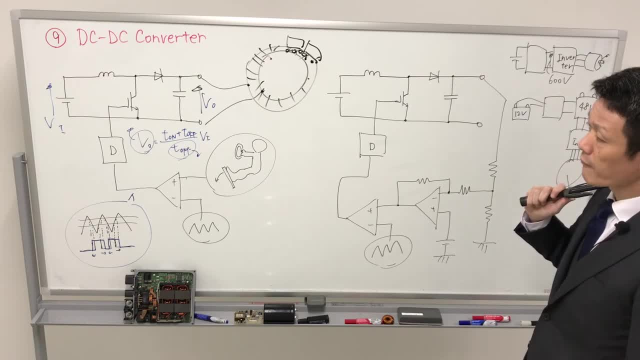 And higher power Around 50 to 100. Over Kilowatt Power. However, In the The real type Automotive area We We must Prepare DC-DC converter, Because the Lower Voltage 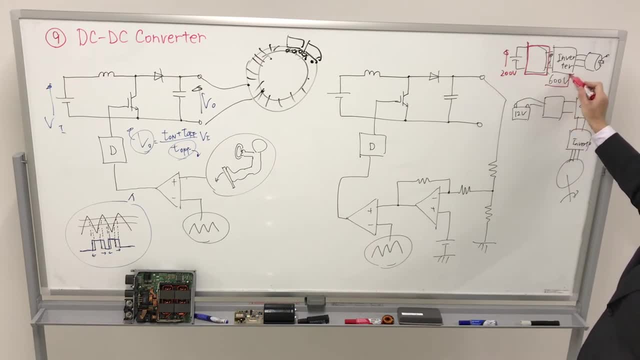 But Inverter side Required Higher Voltage. So Boost chopper is required. One, One Example And Other Otherwise. 20 volt Type, And For Motor driving Required Higher Voltage. 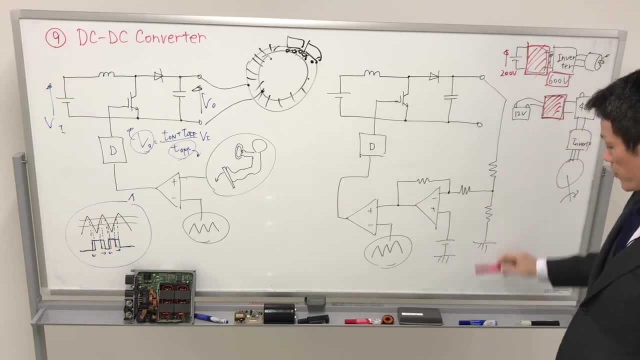 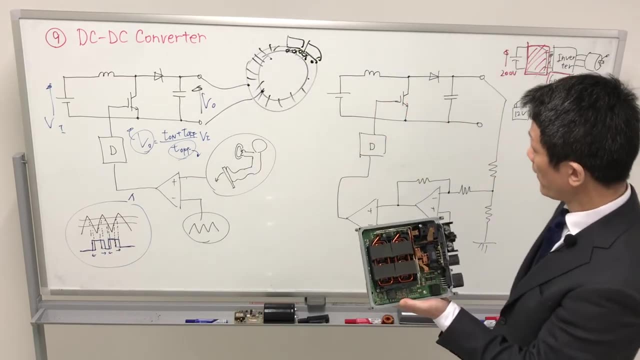 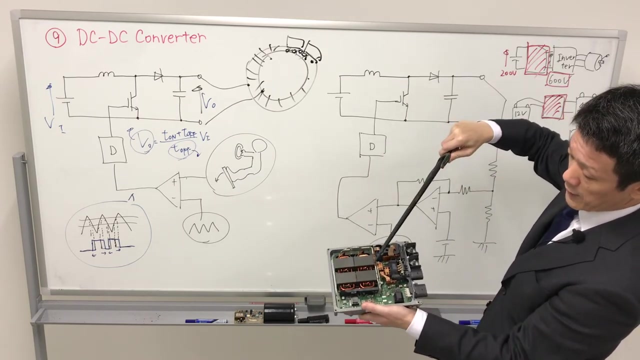 So We Required Boost chopper This, This boost chopper. We Required Hi Sq-7DC DC converter Inductor. Inductor is here. Inductor is The parallel Connect Four Phased. 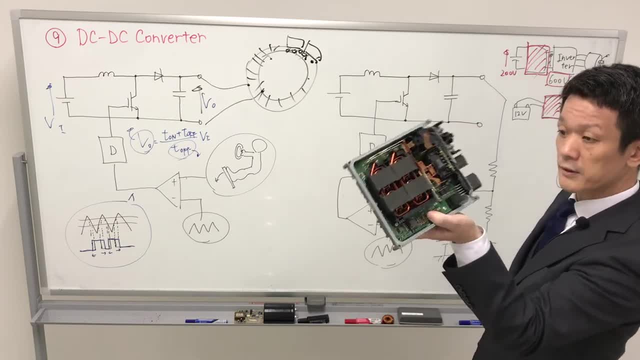 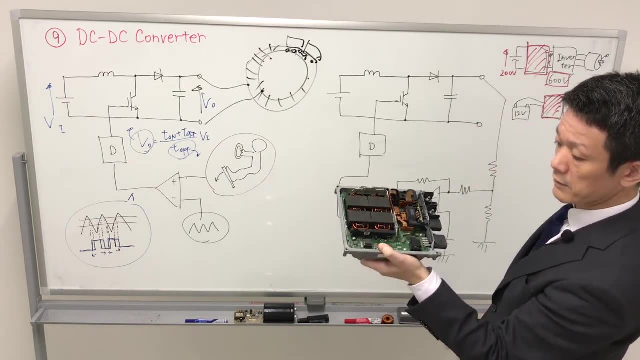 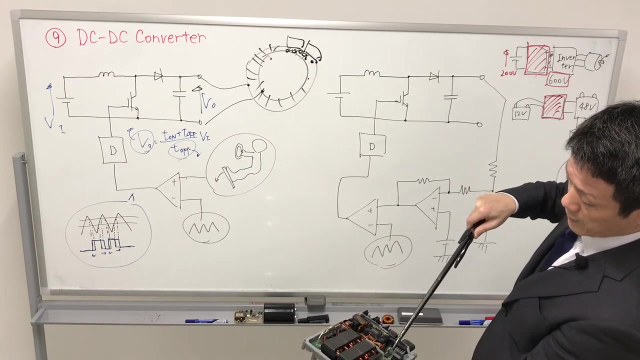 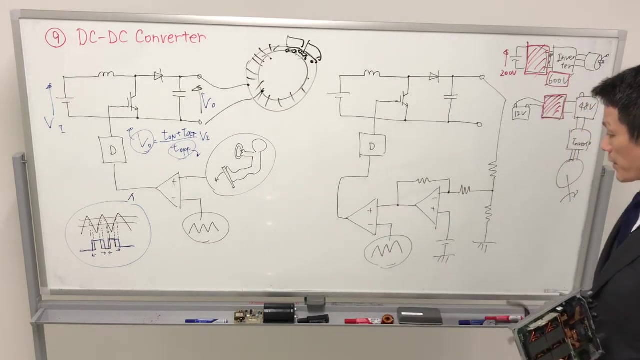 So the Inductor is One, Two, Three, Four For Type Inductor, First The Under This, Under This Inductor And Control here on the opposite side of this PC board, this side here. 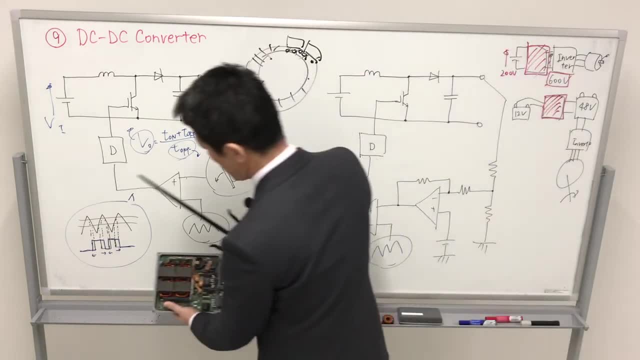 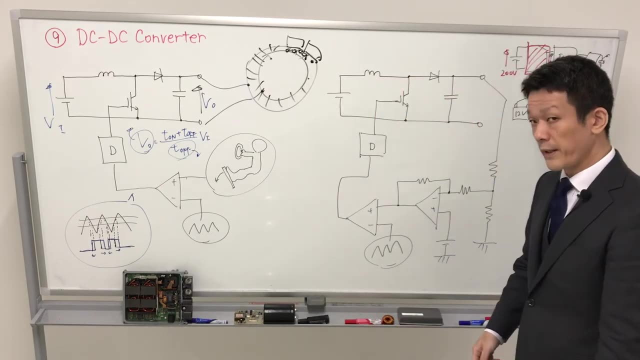 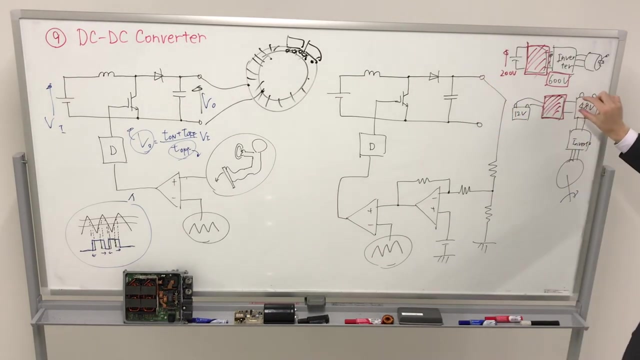 we in the automotive area, the power electronic system, in case of the DC-DC converter, we must obtain the constant voltage for the output voltage, DC-DC converter side. constant voltage required, constant voltage required so that we must obtain, we must prepare for the control side, for the feedback loop. 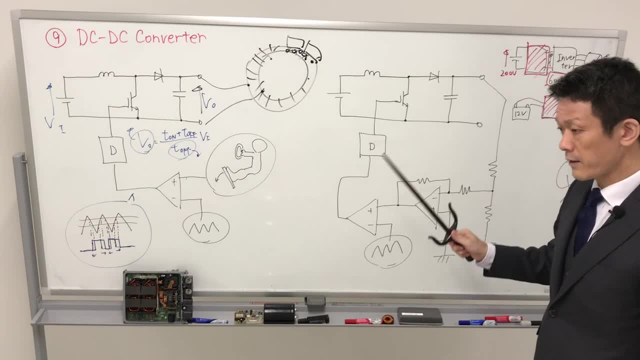 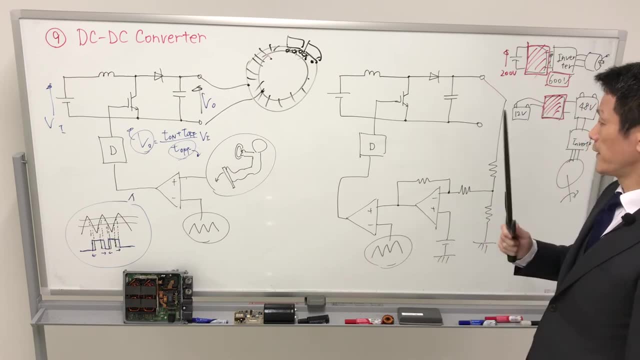 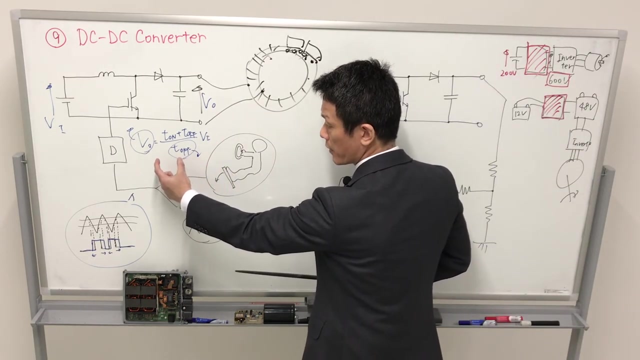 so we must run the feedback control scheme and this is the knowledge ok, and the output voltage increase detection and compare the difference voltage and this is the inverse side, lower side, and compare to this one and lower, higher side that timing is pulse width increase, but the lower side. 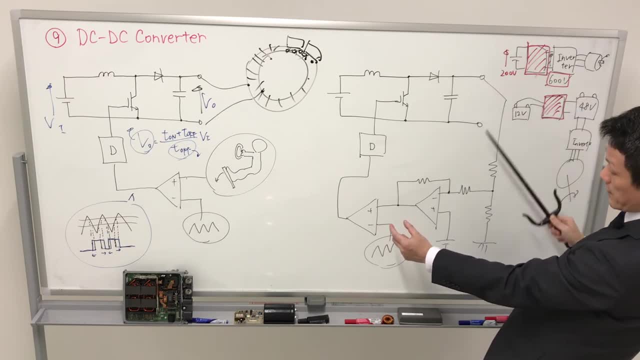 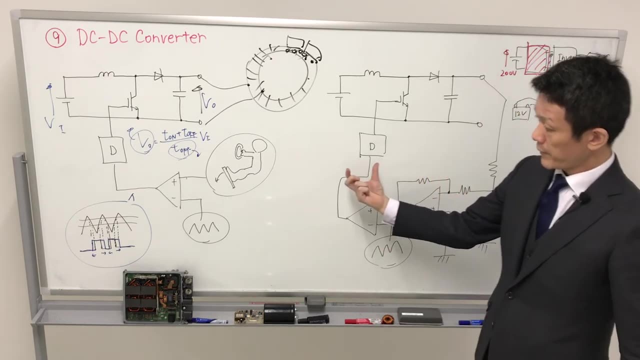 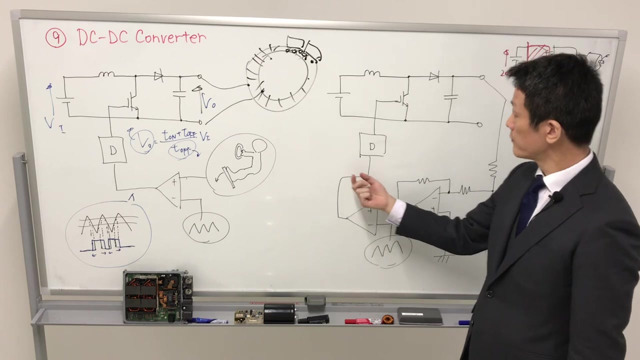 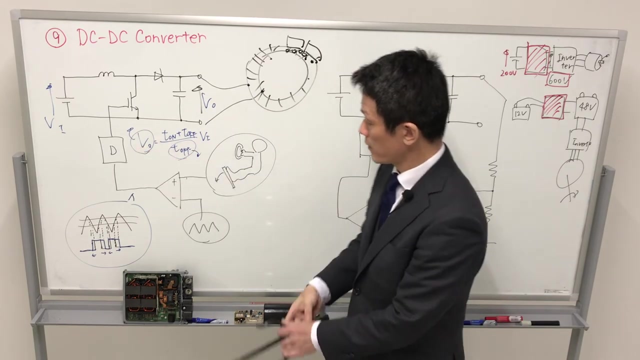 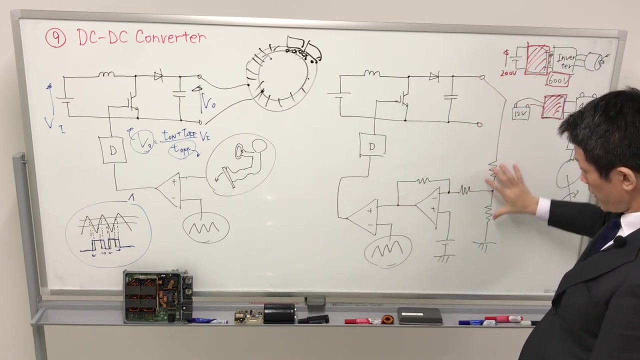 lower side, increase the voltage. this inverse side, decrease, decrease and decrease means turn. T on width is decrease, decrease means lower side because of the decrease and the this one output voltage decrease. so we can keep higher side, this control order: the lower side, higher side, lower side. so we must obtain: